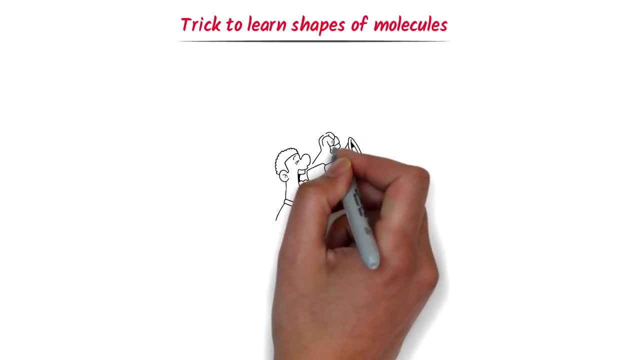 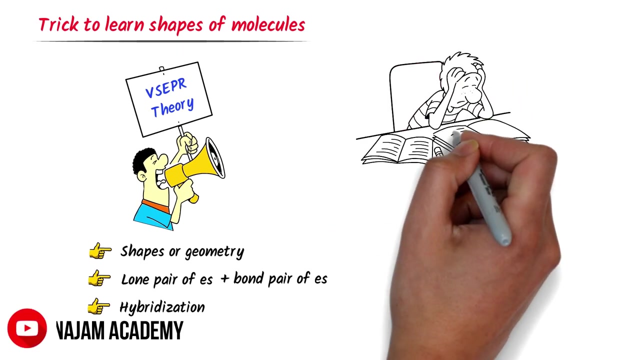 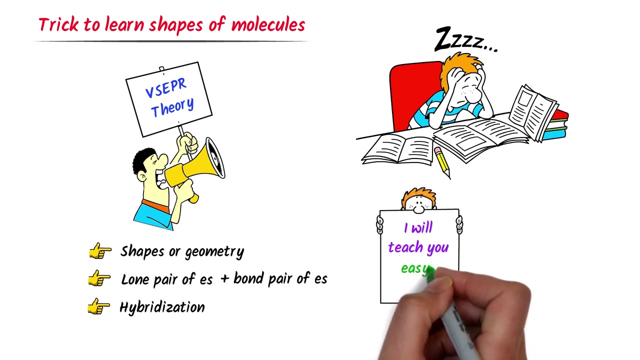 Easy trick to learn shapes of molecules. We know that Whisper Theory teaches us about the shape or geometry of molecules, number of long pair of electrons, number of bond pair of electrons and hybridization of different molecules. Many students find it difficult to memorize the shapes of molecules, But don't worry, I will teach you the super easy trick. 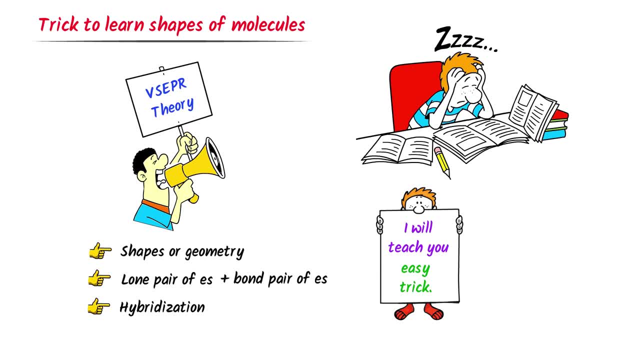 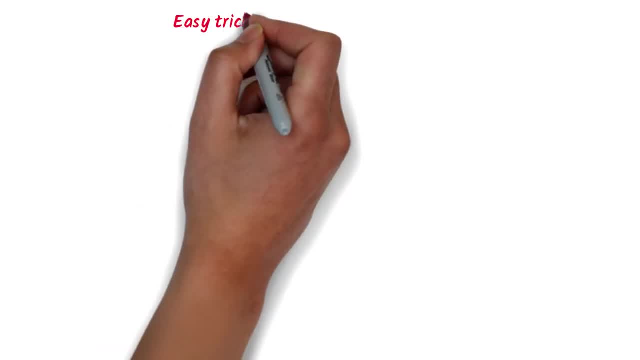 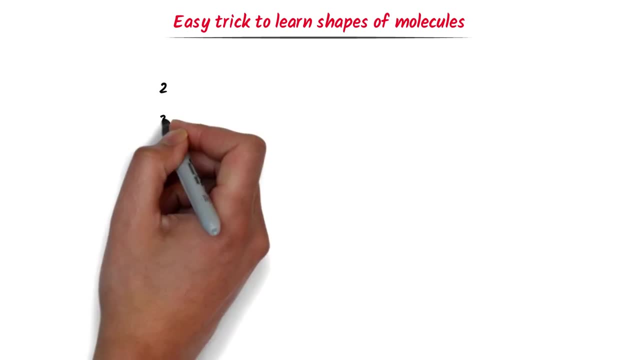 through which you can easily memorize the shapes and geometry of molecules in a very short time. So watch this lecture till the end. Now, what is the super easy trick to memorize the shapes of molecules? Firstly, I write 2,, 3,, 4, 5.. Secondly, I write power for each. 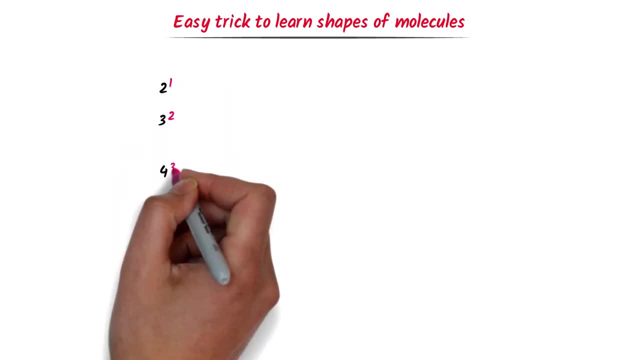 digit. I start from 1,, 2,, 3,, 4.. Now listen carefully. This 1 power of 2 means I have to write 1 times 2.. This 2 power of 3 means I have to write 2 times. 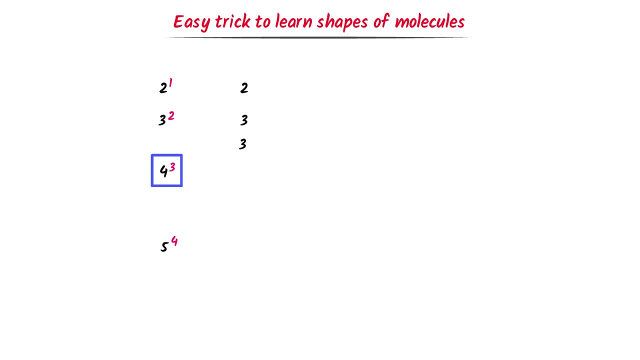 3. This 3 power of 4 means I have to write 3 times 4.. This 4 power of 5 means I have to write 4 times 5.. Thus, remember that power of each digit shows its frequency. Now I write this 2 here as it is. 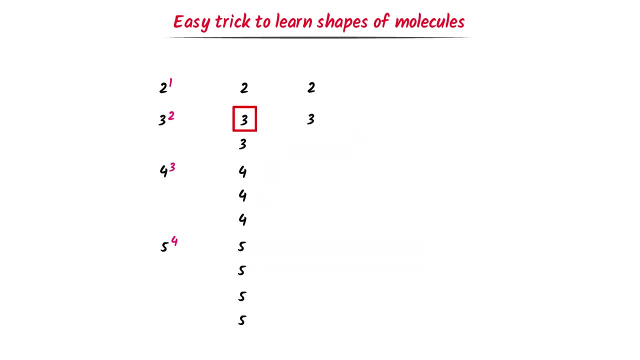 Secondly, I also write this 3 here as it is Now. I go in descending order. This is 3.. I go 1 digit down like 2.. Thirdly, I write this 4 here as it is. I go in descending order: 3, 2.. Fourthly, 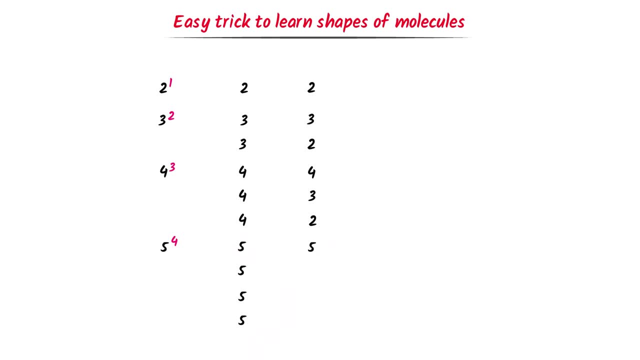 I write this 5 here. as it is, I go in descending order: 4,, 3,, 2.. Lastly, I subtract each row: 2-2 is equal to 0.. 3-3 is equal to 0.. 3-2 is equal to 1.. 4-4 is equal to. 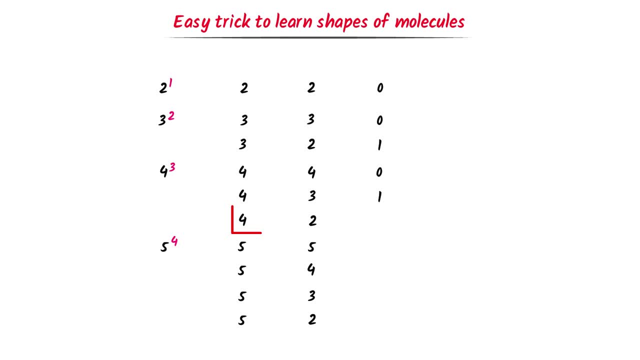 0.. 4-3 is equal to 1.. 4-2 is equal to 2.. 5-5 is equal to 0.. 5-4 is equal to 1.. 5-3 is equal to 2.. 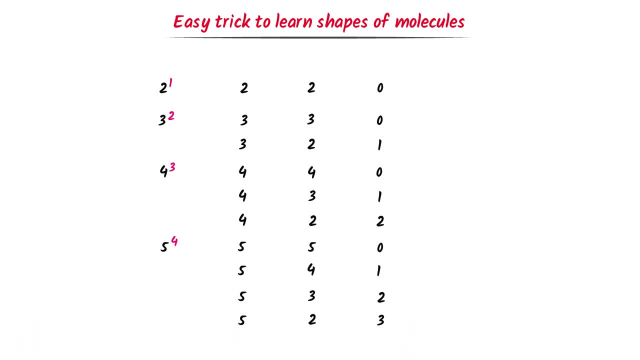 5-2 is equal to 3.. So this column is the electron pairs, this column is the bond pair of electrons and this column is the lone pair of electrons. Thus I have successfully written the 90% code of learning this trick. Now it is time to write their respective shapes. 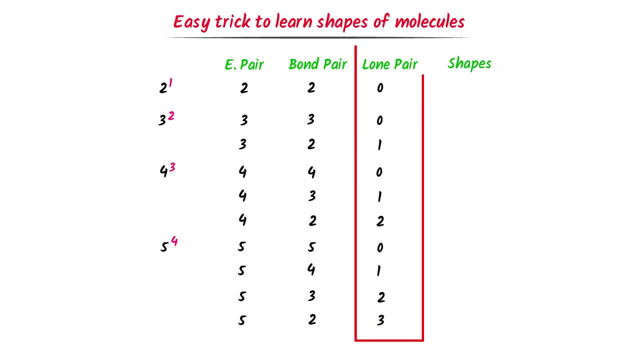 Firstly, I select the molecules having zero lone pair. Let me repeat this important statement: I select all the molecules having zero lone pair, For example, this one, this one, this one and this one. Now listen carefully: If bond pair is 2,. 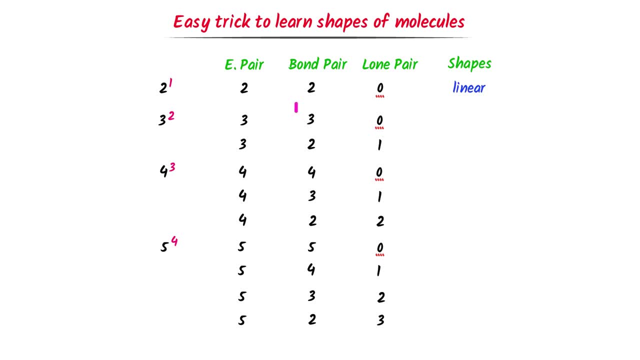 it is always linear. Secondly, for this three, I write trie. For this four, I write tetrah. For this five, I write trie, which means 3, and I write bi, which means 2.. So trie plus bi is equal to 5.. Now listen carefully. This trie stands for trigonal. 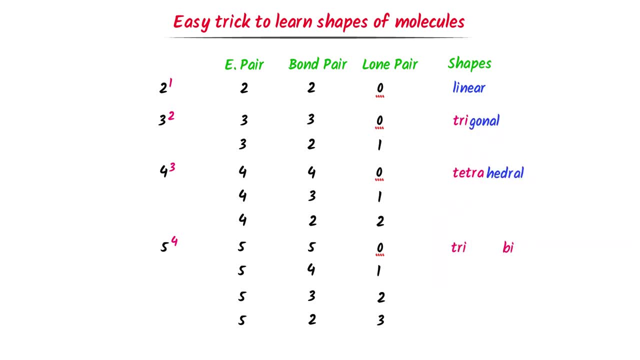 This tetrah stands for tetrahedral, This trie stands for trigonal and this bi stands for bipyramidal. So these are the shapes of molecules having zero long pairs. Now what about the shapes of other remaining molecules? Well, I teach my personal mnemonic. 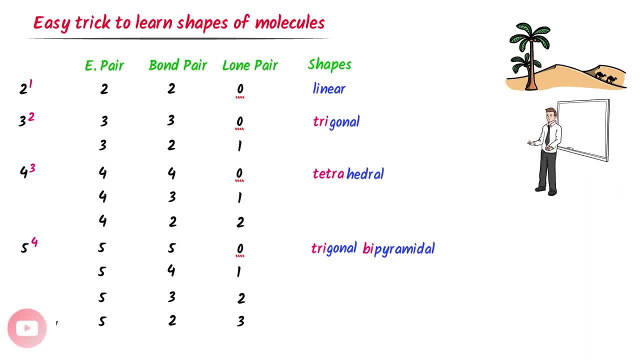 Consider that your SS teacher live below a top valley. I say: below top valley SS teacher live. Let me repeat it: Below top valley SS teacher live. Now, this ben below stands for bent shape, This tp and top stands for trigonal pyramidal. 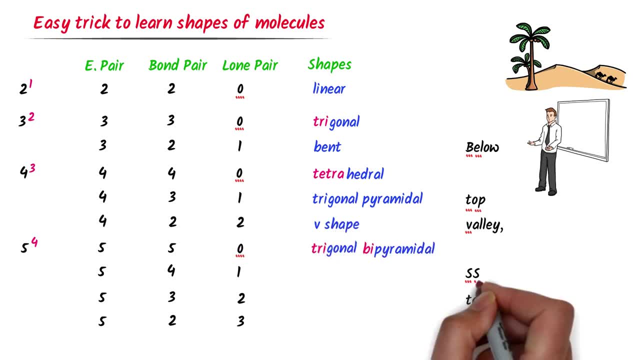 This v and valley stands for v shape, This ss stands for seesaw, This t and teacher stands for t shape And this li and live stands for linear shape. Thus, using this simple trick, we can easily memorize the shape of molecules. 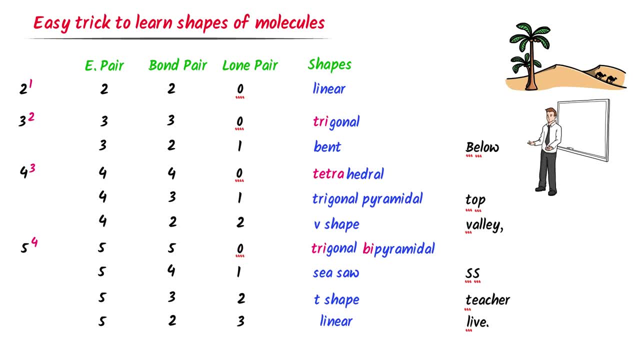 Lastly, let me teach you that how can we use this trick to draw the geometry of any molecule? Well, consider this case. Let the central atom is a. I draw two bond pairs like b, And we know that it has zero long pair of electrons.